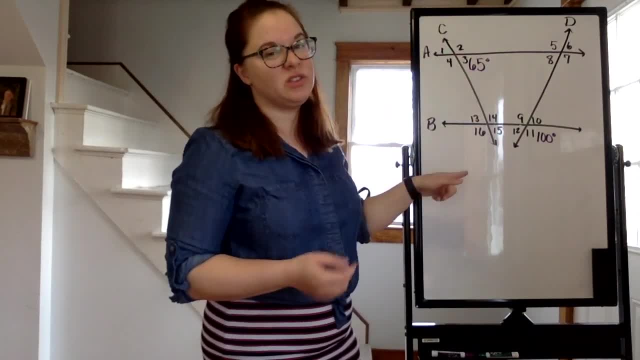 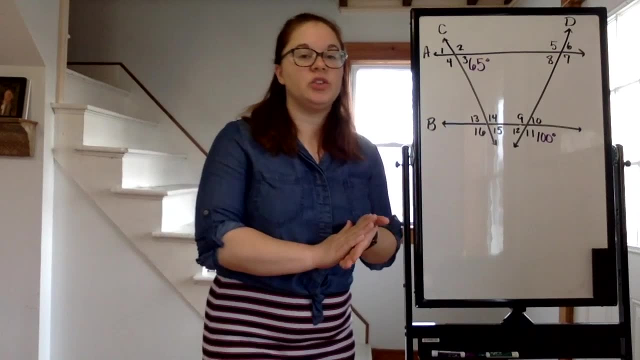 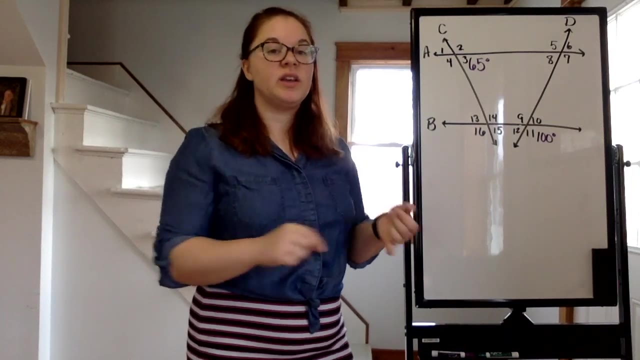 on the angle measures for transversal C. So we're going to pretend that this half does not exist. So let's start looking for some easy angle measurements. we can know We're going to use corresponding angles and vertical angles. So in red I have my corresponding angles, I know. 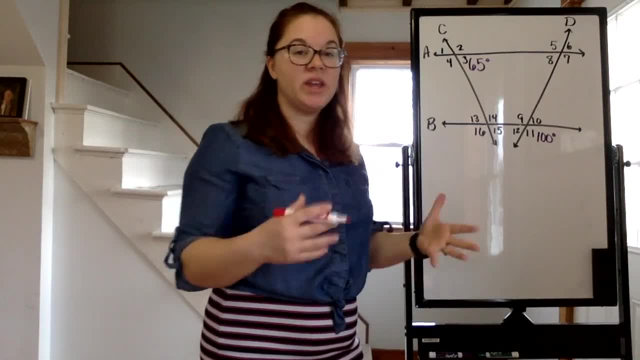 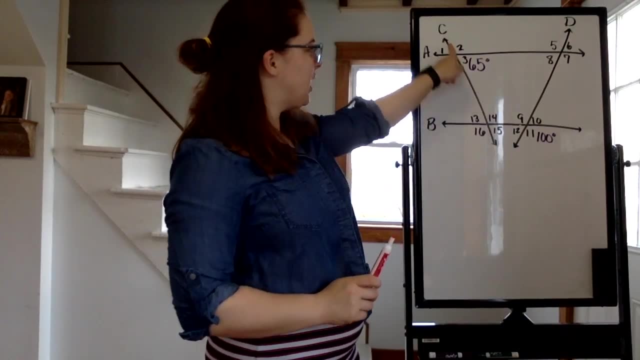 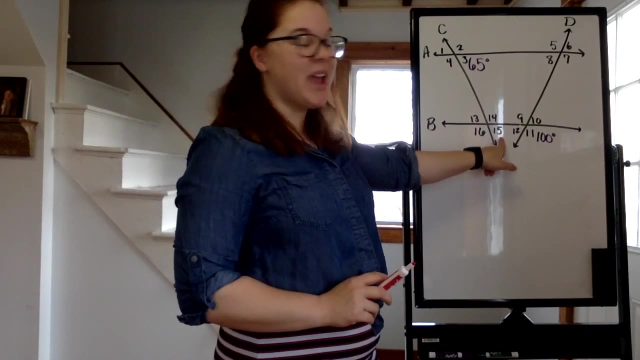 that angle 3 is in the bottom right hand corner of this transversal right Here. so I'm going to go to the second place where line C transverses that other parallel line. I'm going to go to that bottom right hand corner and I know that angle 15 is also 65 degrees. So 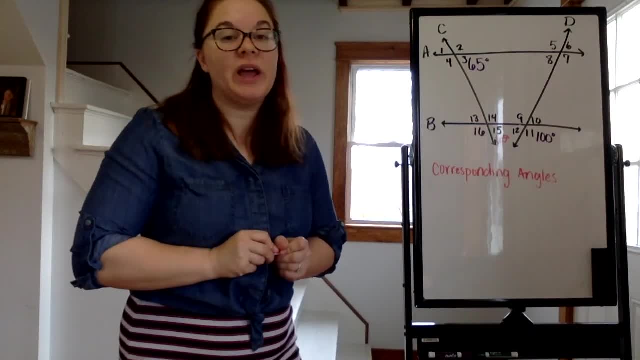 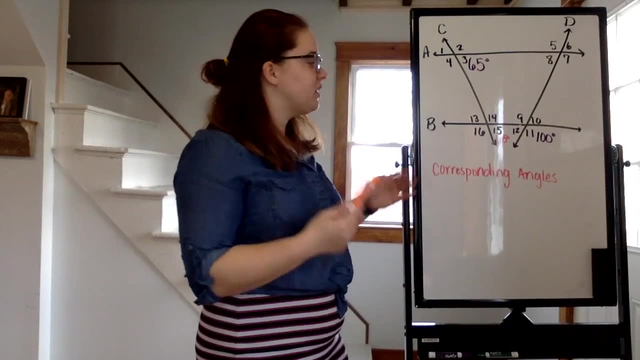 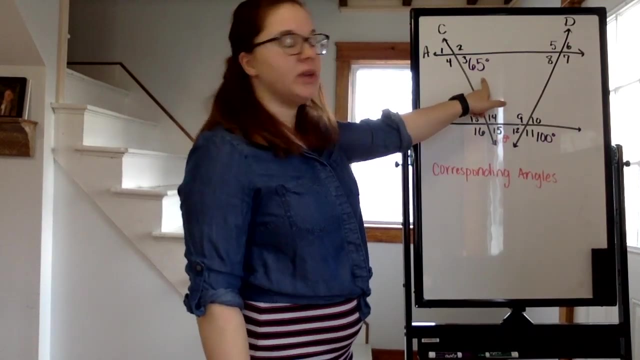 now I can use vertical angles to figure out two more angles. So we can now use vertical angles- I'm going to mark them in orange- to find two more angle measures. and remember vertical angles are congruent with one another. So angle three that we were given at the beginning is 65 degrees. 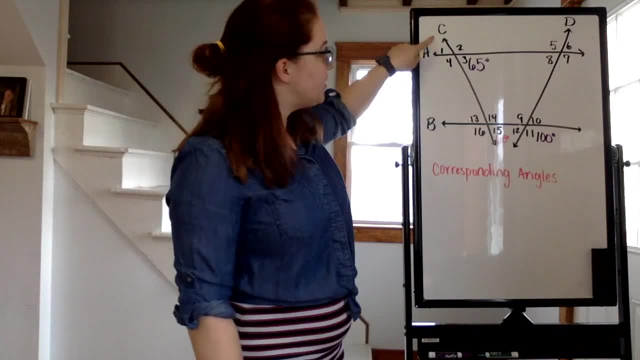 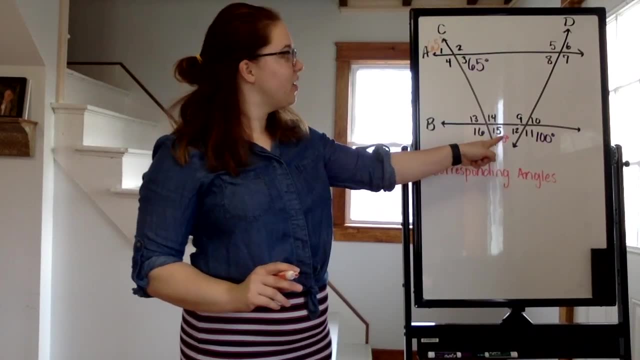 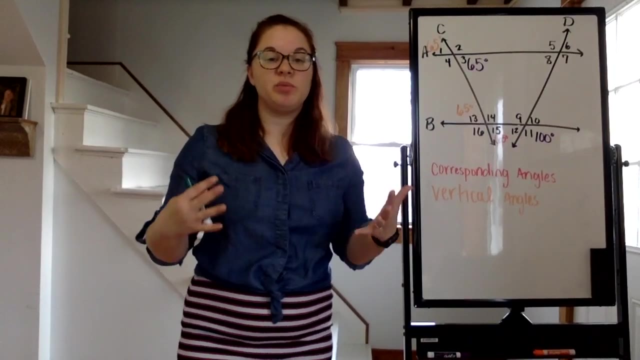 is composed of these two lines, and so is angle one. So angle one is also 65 degrees and again, working with transversal C, we can see we have another vertical angle, Angle 13,, again 65 degrees. So now we're going to use some other principles of angles that we know. 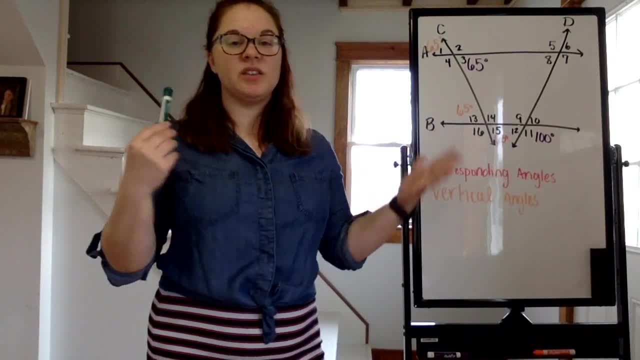 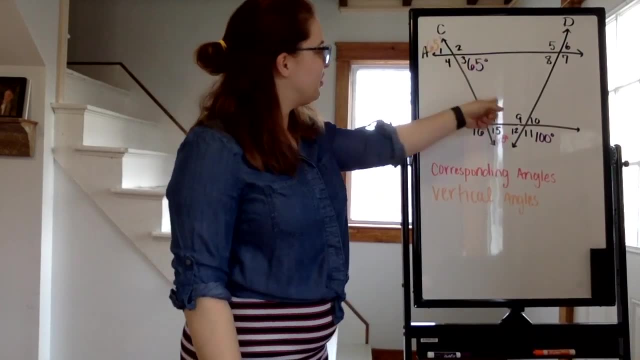 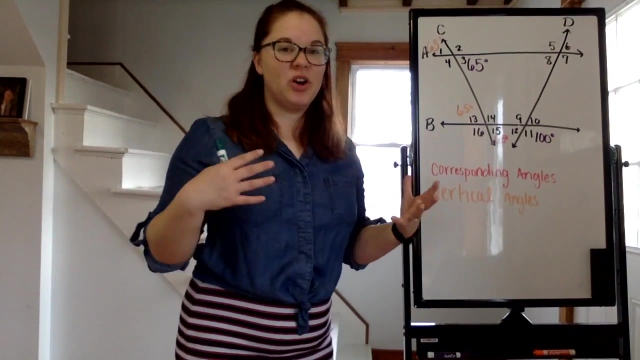 angle relationships. We're going to be using supplementary angles And we're going to use angles that make up a straight line to figure out what these remaining angles are. And the really cool thing is we know that these angles are all going to be the same size, right? Because 65 plus. 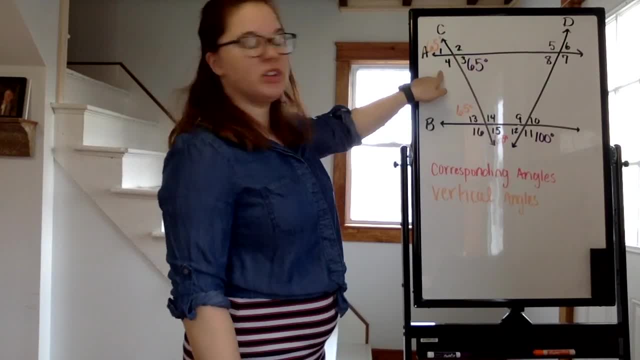 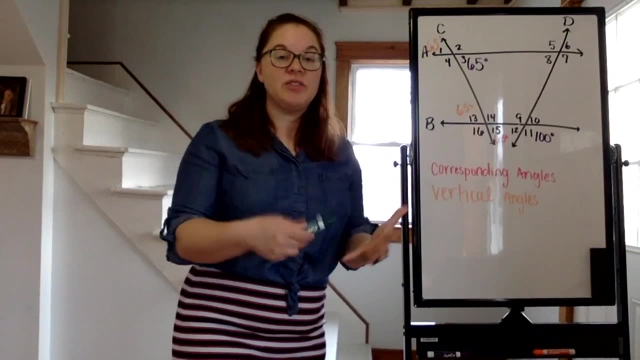 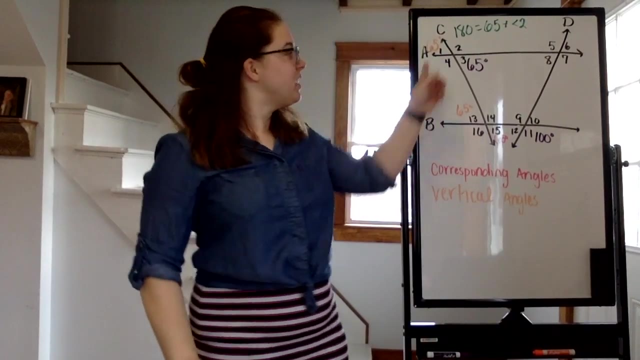 something is 180 and that is vertical. with that, This is a corresponding angle here and this is a corresponding angle there. So we just have to do the math just the once to figure out what the rest of these angles are. So we know, because these are supplementary, 180 degrees is. 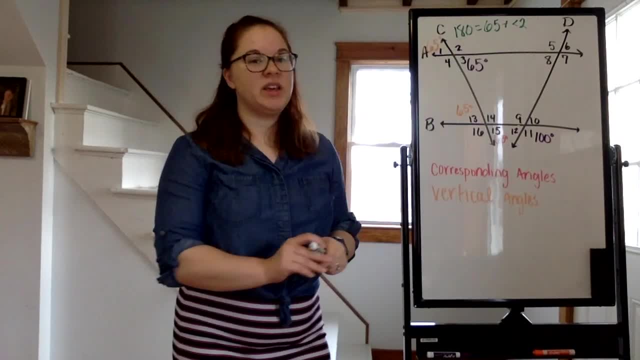 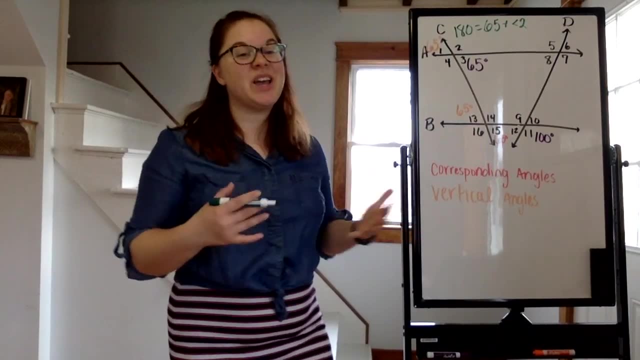 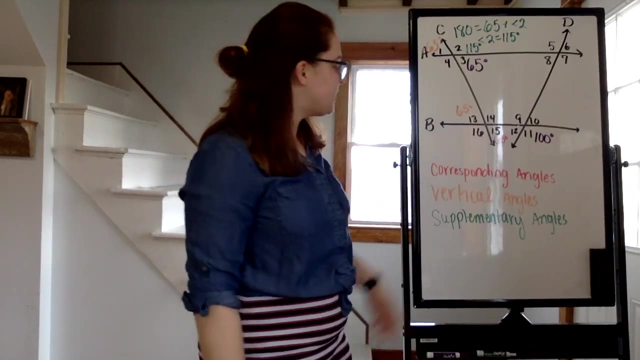 this 65 degrees, plus whatever angle two is. If we solve that algebraically, subtract 65 from both sides, we know that angle two is 115 degrees. So now that we've found angle two, we know the rest of these angles. We know its corresponding angle, Angle 14, is also 115 degrees. 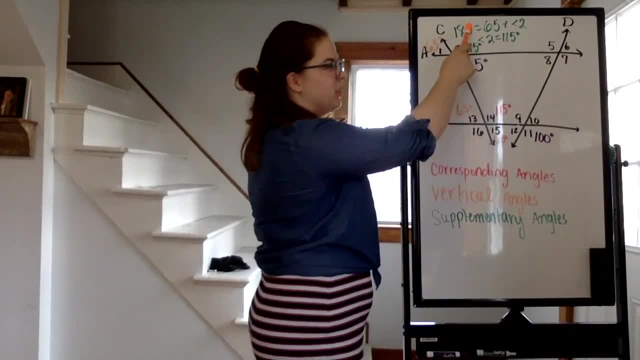 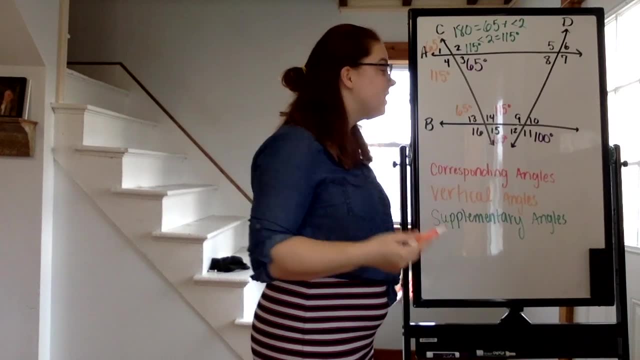 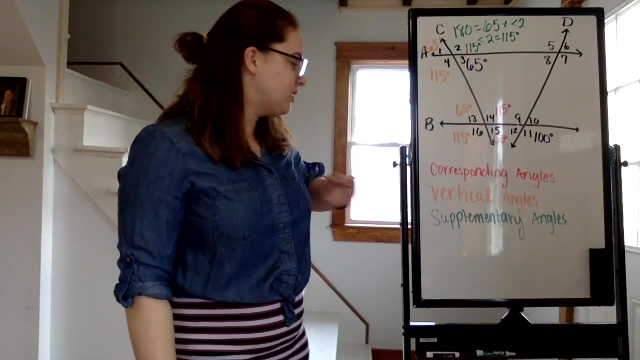 We also know that the vertical angle to number two, angle four, is 115 degrees, And we know the vertical angle to angle number four- angle 16, is also 115 degrees. So, just using these three types of angles- corresponding angles, vertical angles and supplementary angles- using those, ideas, we were able to solve all of these angles in transversal C. I'm going to clean this up Because we've already solved for transversal C to work on transversal D. I'm going to keep this same color code because it's really easy to be able to spot how we could use corresponding vertical and. 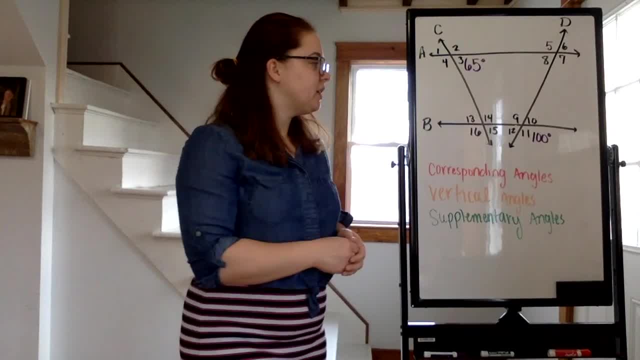 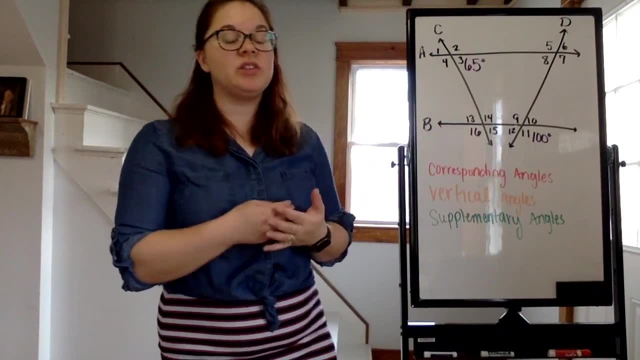 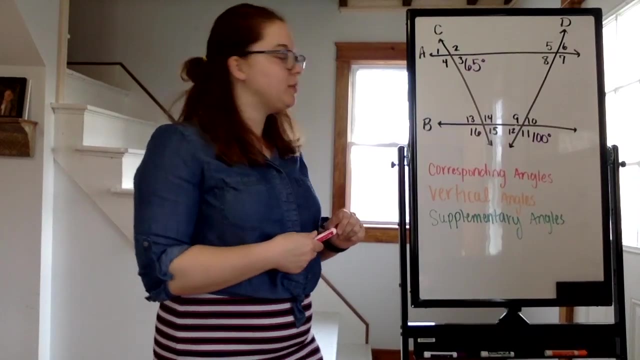 supplementary angles here. So I am given one angle measure and that's angle number 11.. So what I'm going to do is I'm going to start by looking for a corresponding angle to angle 11. Our corresponding angle here It's going to be in that same lower right hand corner and that it's going to be on. transversal D. This time we're going to ignore transversal C, like it's not there. So our corresponding angle to angle 11 is angle number 180.. We can go side to side, We can go up and down with linear pairs. It doesn't matter if you go. So at the beginning we were given 11, which is 100 degrees. Well, if 11 and 10 are going to add up to can go through, use bonding or they're vertical. So there you have it. So we're starting out with a new example and we have a bunch of lines L, M, N, P and Q and transversal T. So we're going to start by adding the known angles that. we're given in the problem. So here we're given L, M, N, P and Q. So we're going to start by adding the known angles that we're given in the. So here we're given L, M, N, P and Q and transversal T. So we're going to start by adding the known The angle needs a line. So we're going to use the types of angle relationships we know: Linear pairs, vertical angles, complementary angles, supplementary angles, corresponding angles- through what line is parallel with this top one. So I'm actually going to underline this. one with another color. So remember, this is our frame of reference. You're trying to figure out what is parallel to line L, So we're going to use what we know about it. There are some rules, So we know that when a line transverses two parallel lines, it's going to create corresponding. angles. So the idea of corresponding angles is that when we have an angle, this upper left-hand corner of the transversal. that means that where this line T transverses a parallel line, it will have an angle of the same measure, congruent angle- in the upper left-hand corner. So let's check it out. So we've got our upper left-hand corner is 110 degrees. So it's not possible that this one is parallel And because we're working with a whiteboard, I'll just erase this one because we know it's not parallel. So line M: is not parallel. What about line N? Well, this should be 120 degrees and that's only 100.. They're not parallel lines. Line L and N are not parallel, Otherwise this upper left-hand angle would be 120 degrees. So we can get rid of this one too. Sorry, line N, you are not parallel to. line L. Now let's look at line P. Well, on line P we don't have that corresponding angle, so we're going to skip it for now. Now let's look at line Q. This corresponding angle, the upper left-hand, is 60 degrees. 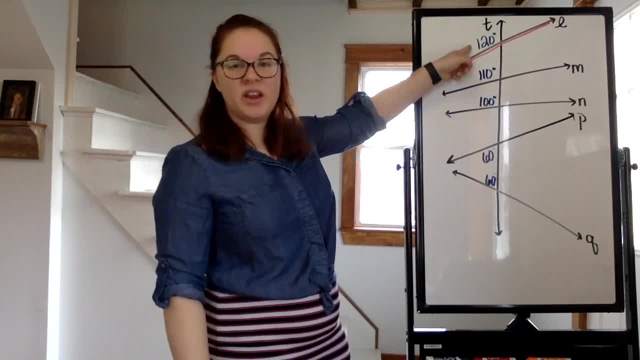 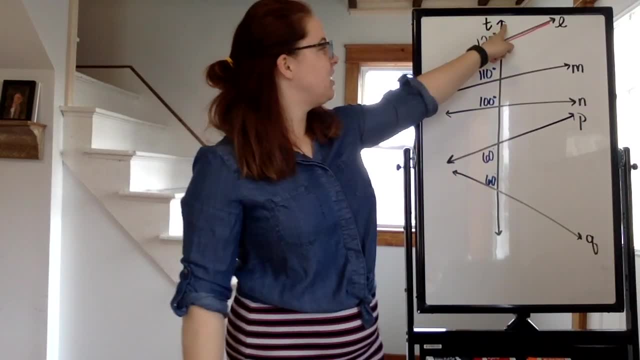 where this one is 120 degrees. Okay, this one can't possibly be parallel, Sorry. line Q. Well, now we're left with line P, and we know that it may be parallel, but maybe none of these were parallel to begin with. 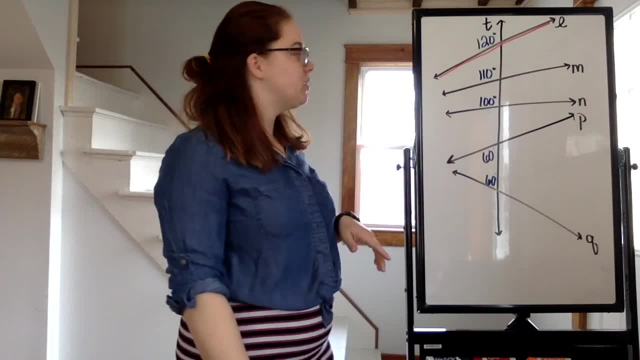 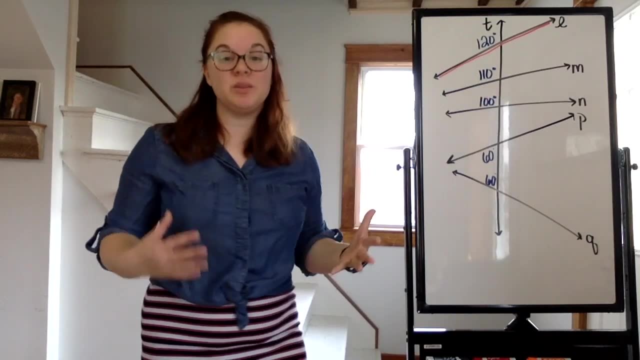 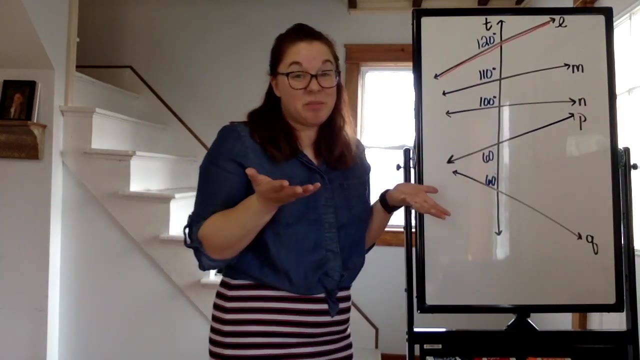 So what we can do is we can use another kind of angle. What we can do is we can use another kind of angle pair to figure out if line L and P are parallel. So if we look at this, they're not corresponding angles given. so you can actually use what you know about angle relationships to 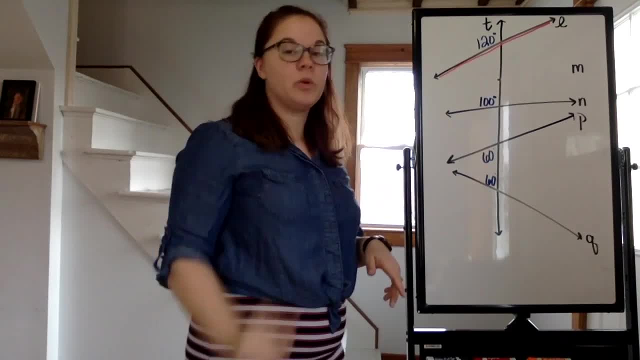 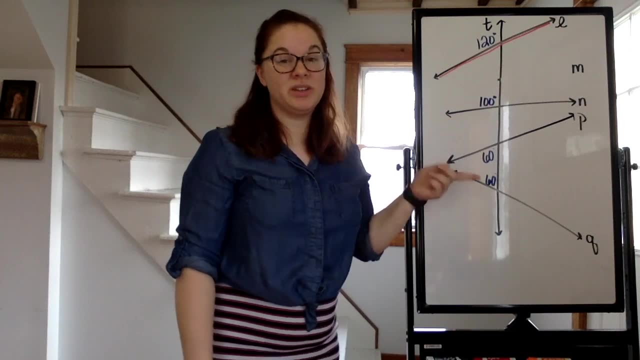 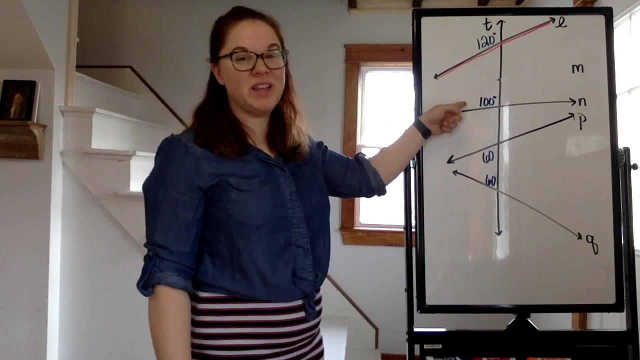 get a little bit more information on the angles where T meets line L. So I'm going to add what I figure out in light blue. These are my calculations, So I'm going to use the idea of supplementary angles to figure out what these other angles are. 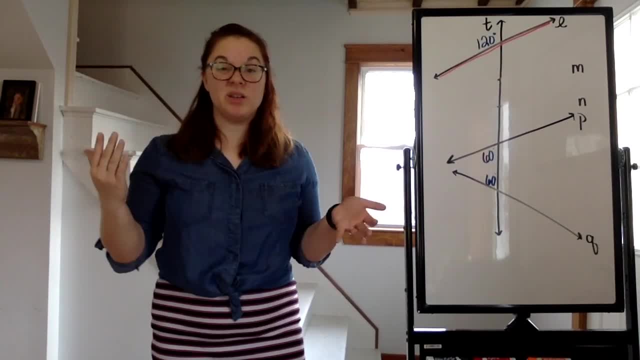 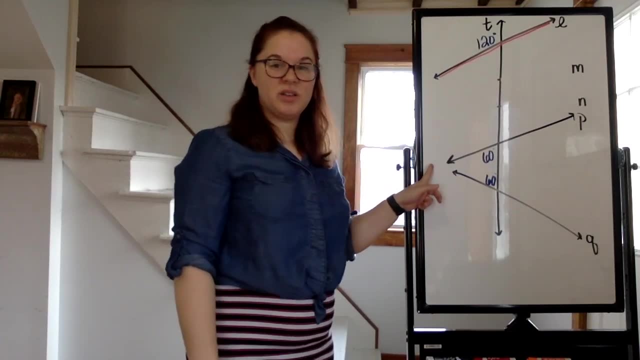 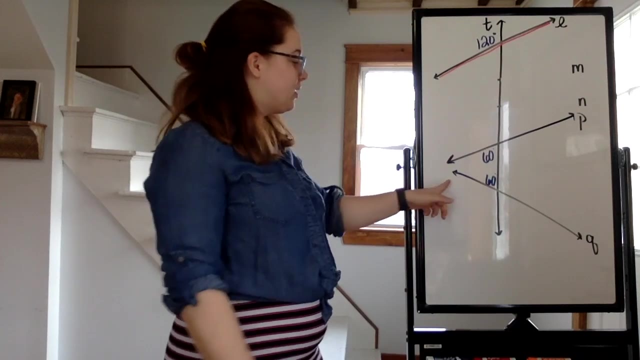 So I know that this angle and this angle have to add up to 180 degrees. So if this one is already 120, this angle here is another 60 degrees, And I'll just go clockwise to figure these out. Well, I can use vertical angles to figure out this one. So this angle is 120. 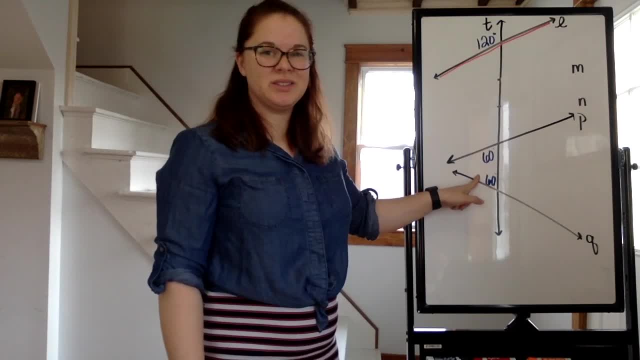 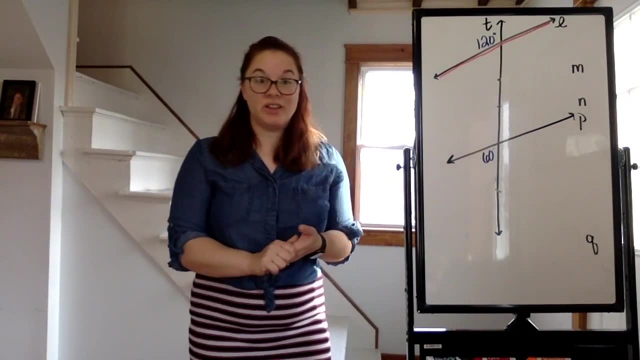 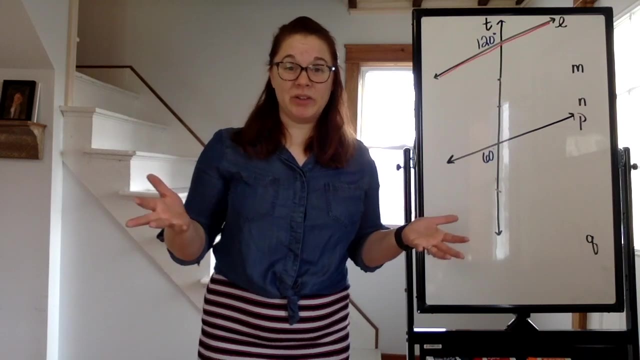 And I can use vertical angles here to figure out that this angle is also 60 degrees. So now let's check back in with line P. Well, oh wow, we have a pair of corresponding angles. So we know that these are parallel lines, And we can prove it by doing the same process here, using supplementary 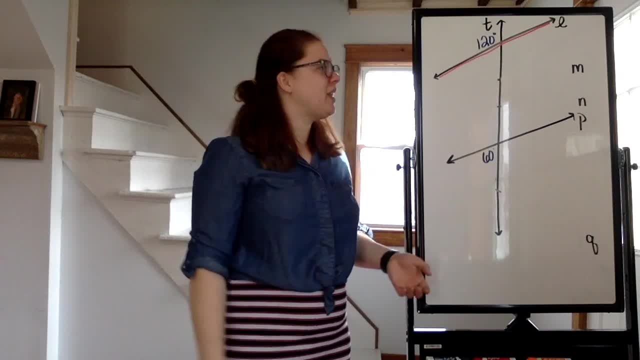 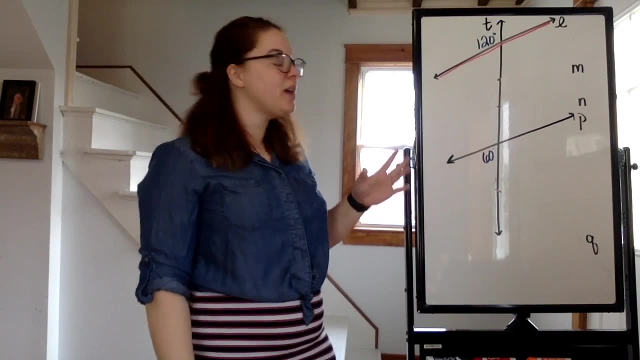 angles, using vertical angles to find the rest of these angles to show that these are parallel. they do have the same four angles. So this is our last example. It's a parallelogram, it's got some given angles and it looks so different than the other transversals. 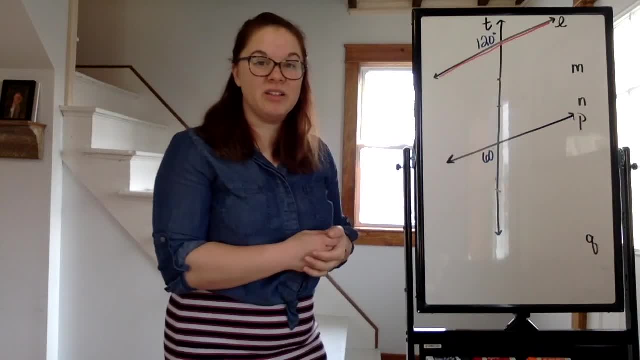 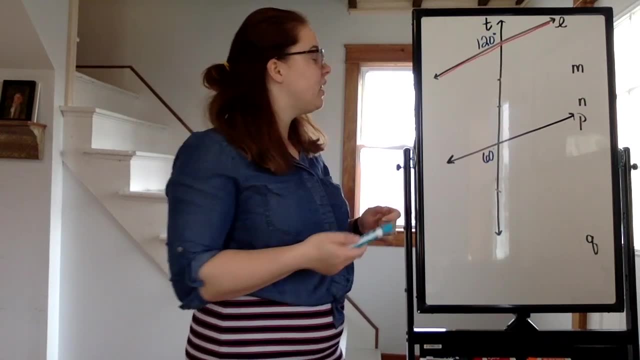 we've been working with, but it's not that different than our first example. So what we can do is we can actually extend these lines to make it look more familiar. So this might look a little messy, but we can start to use some of the angle relationships. 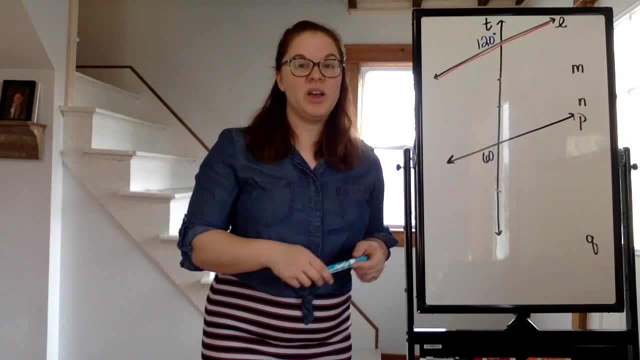 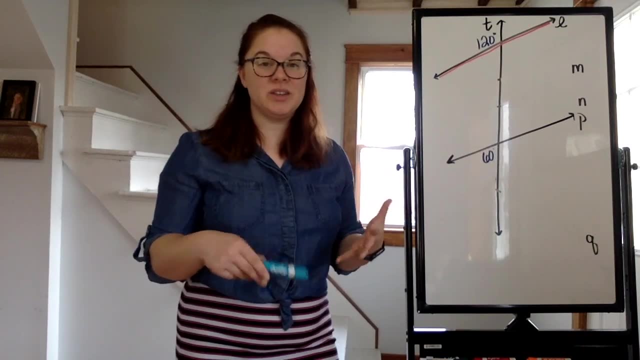 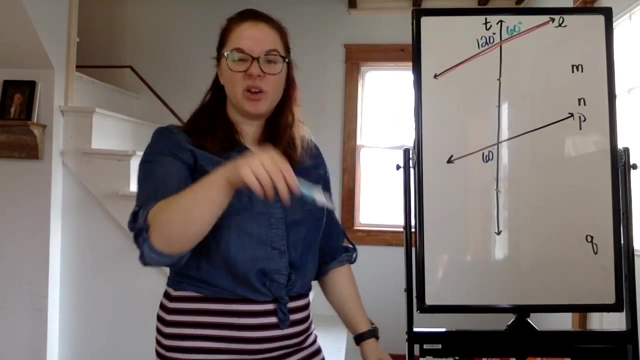 that we know that are easy to work with, to see if we can figure out some of these additional angles. So I'm going to start with some corresponding angles because I find them really easy to work with, So we can take this transversal here. 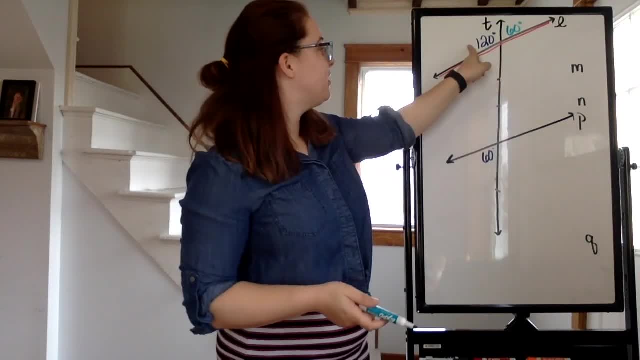 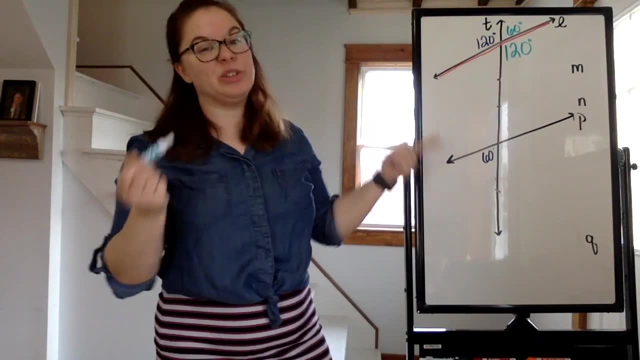 It's a little crooked because I'm not an amazing artist, but you get the picture. This, in an ideal world, would be a straight line. I know when this line meets one of these parallels, it's gonna create a 37 degree angle. 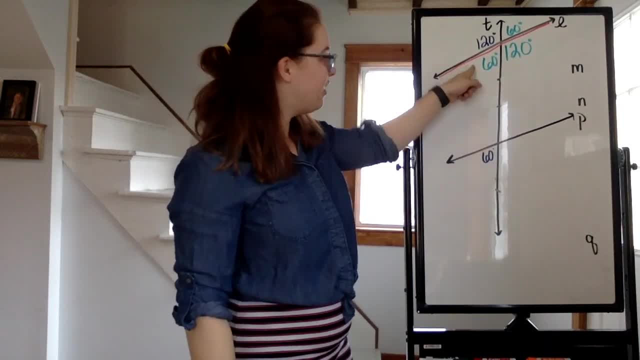 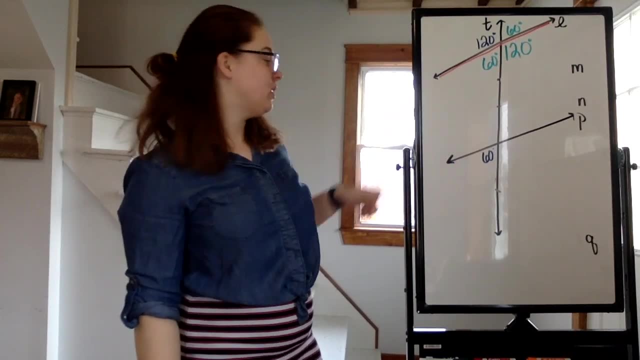 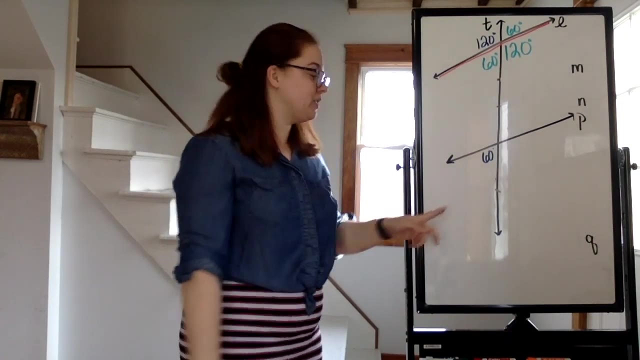 So I know that this here is 37 degrees, this will also be 37 degrees. I know that when this line, this transversal, hits this parallel line, it's 76 degrees. Here's that other parallel line, so this one must be 76 degrees. 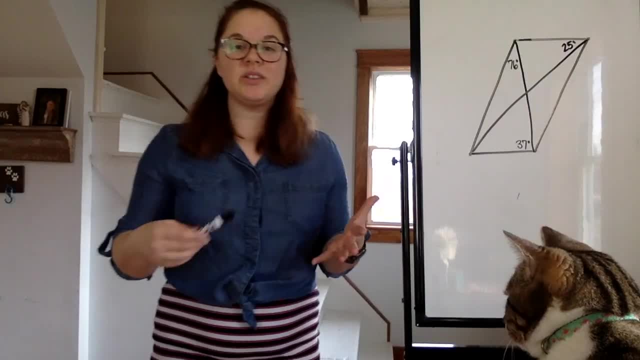 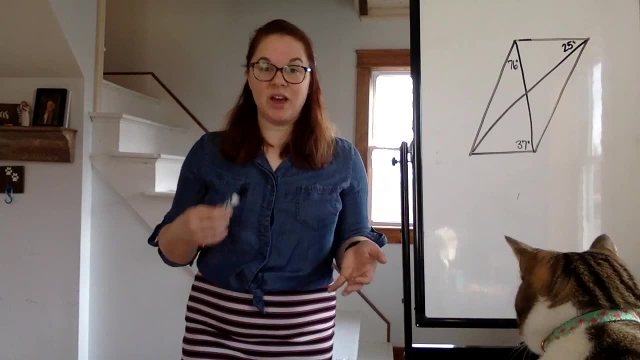 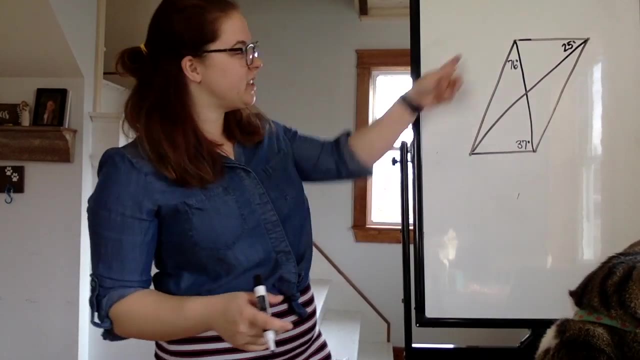 I then can use the idea of vertical angles to figure out a couple more angle measures. This shares the lines that make it up with this angle, so they're both 76 degrees. I can then use vertical angles on those 37 degree angles, and this angle shares its. 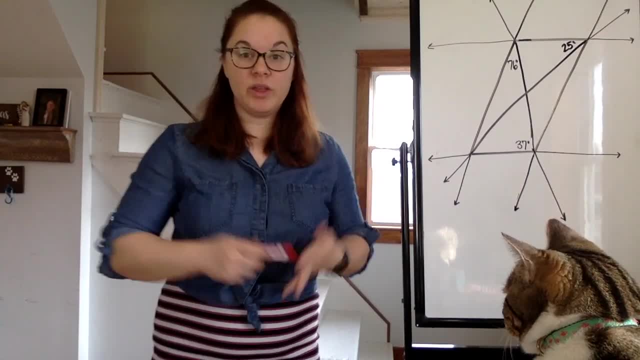 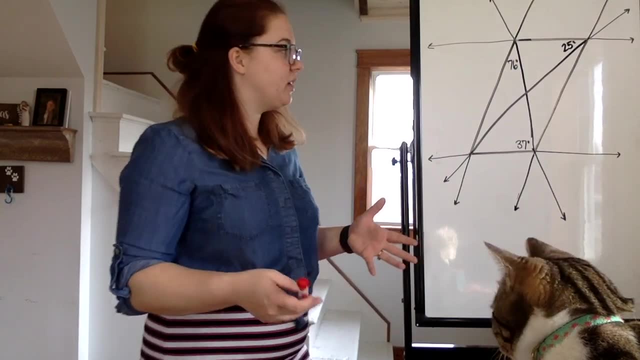 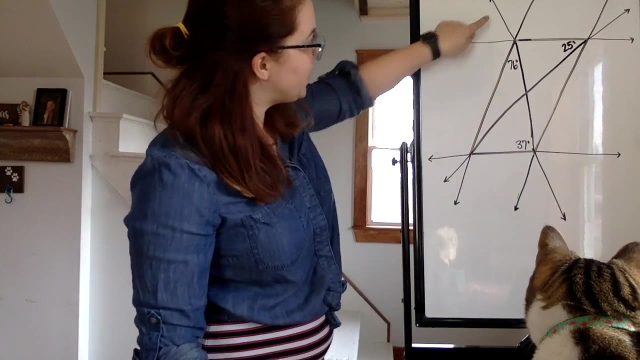 lines that make it up with that angle, so that's 37 degrees. and this angle is a vertical angle with this, so that's also 37 degrees. So, finally, we can use the idea of supplementary angles to figure out the last angle here. So I know that. 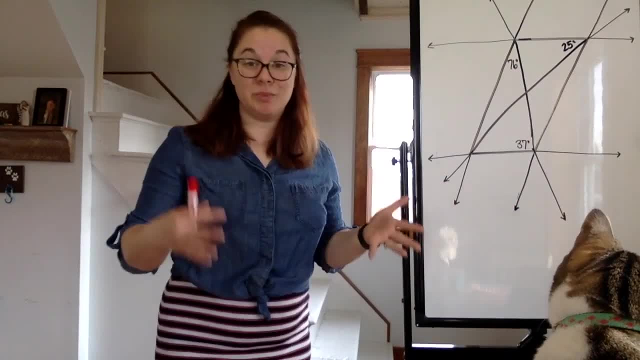 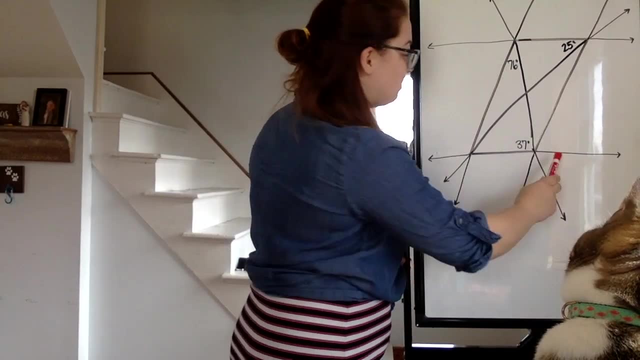 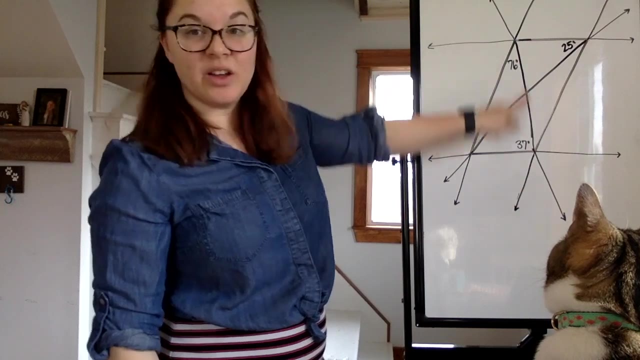 these three angles together are 180 degrees, So I'll use a little bit of algebra to solve it. So I know that 180 degrees equals 37 plus 76 plus whatever this is. So I can use some algebra to figure out that this unknown angle is 67. 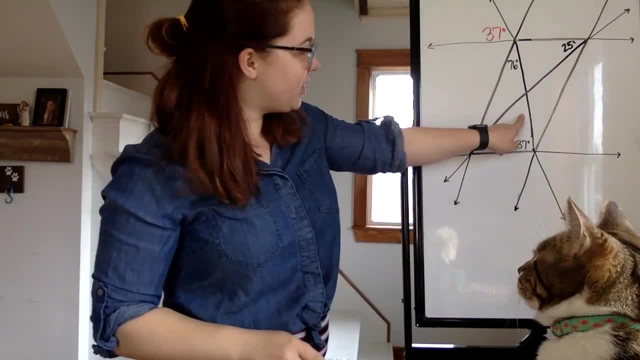 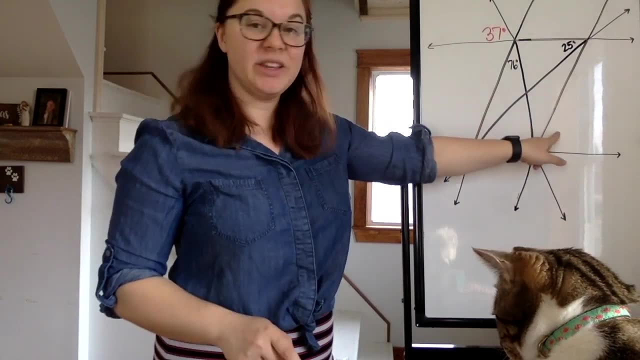 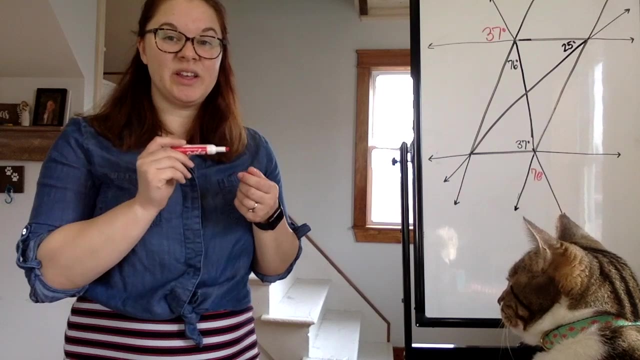 degrees. I then can use a corresponding angle to know that this is also 67 degrees. Then I use my vertical angles to find these two measures, also the measure of these angles. So let's start with our least defined- I know when- this 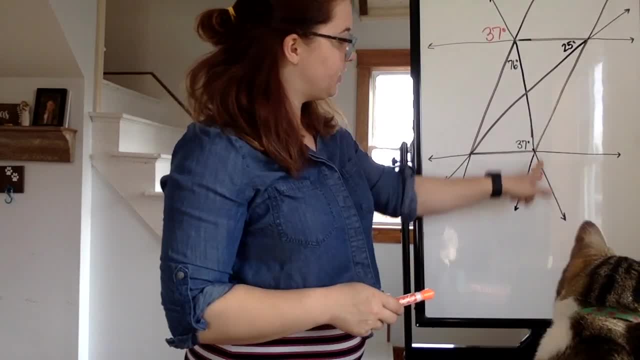 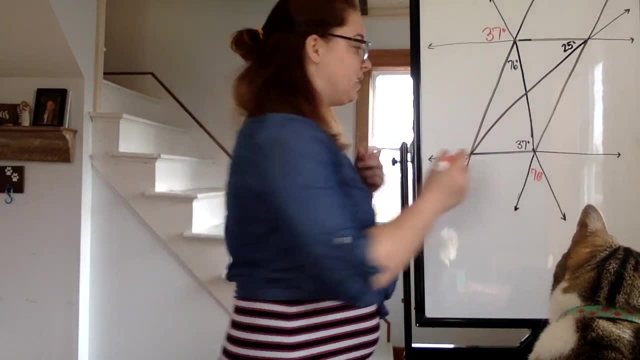 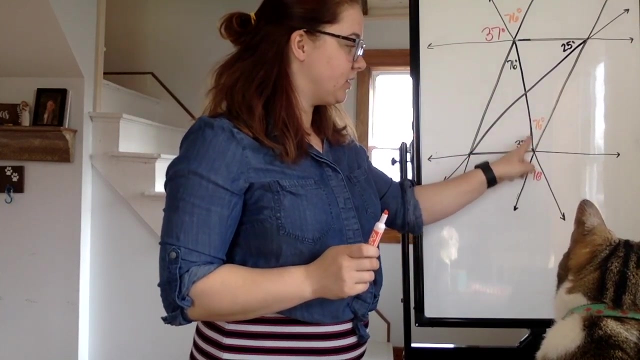 transversal here, that lower angle, 25 degrees. I then use a corresponding angle to find about 75 degrees, and this transversal here is 23 лучes, I know when. then use vertical angles if I can. So this must be 25 degrees the measure of these. So in order to 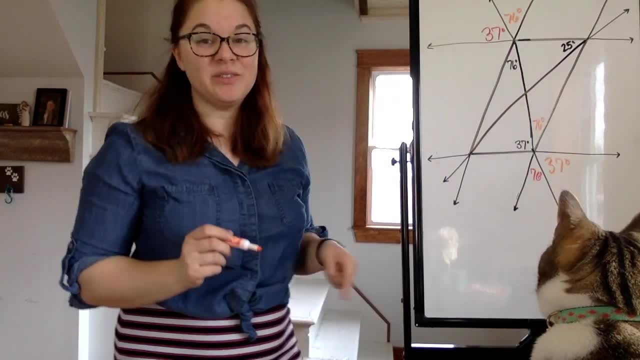 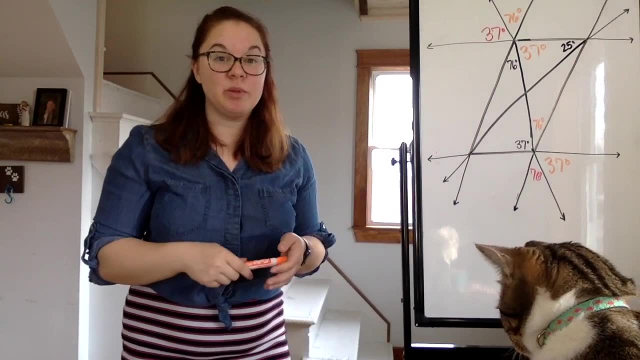 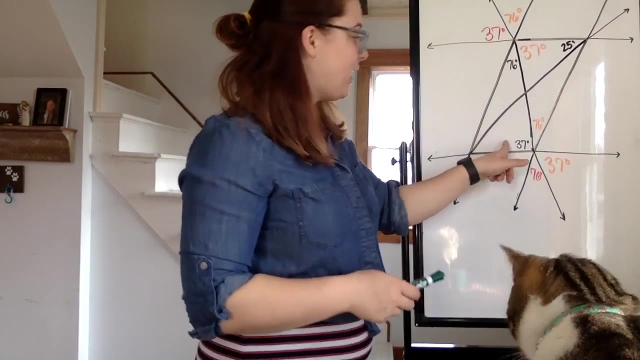 find those last two angles. we need to remember something about four-sided figures. For four-sided figures, like squares or rectangles or parallelograms, their angles on the interior are always going to add up to 360 degrees. So now what we're going to do is we're going to figure.